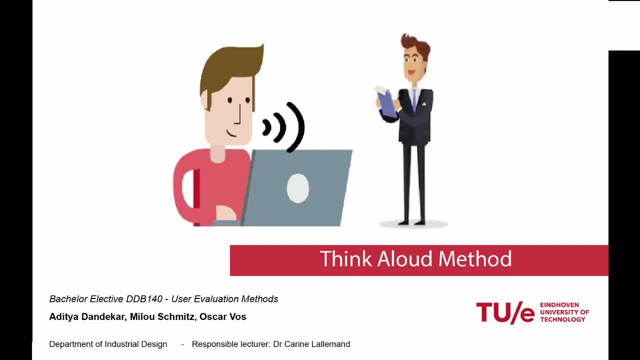 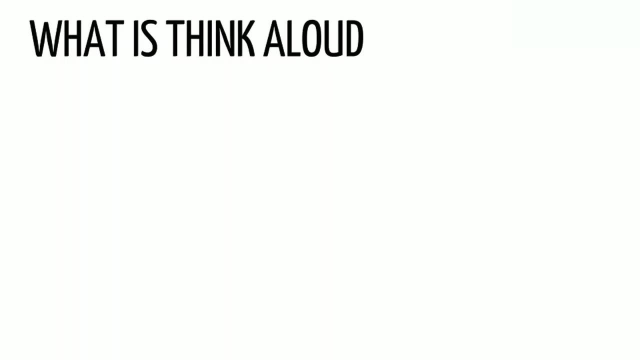 Today we are going to talk about the think aloud technique, which is a usability testing method. The think aloud technique, also called think aloud protocol or verbal protocol, is a qualitative data collection technique. It is a technique where participants speak out what is going on in their 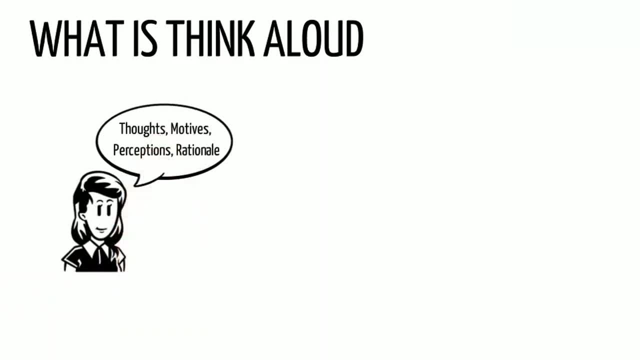 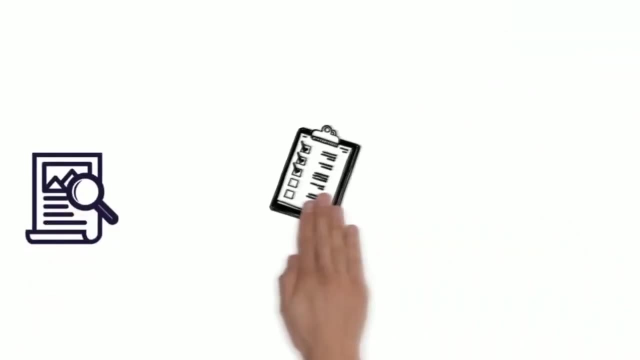 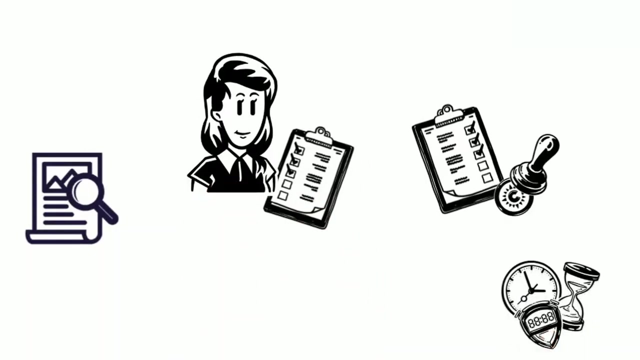 mind, including their motives, rationale and perceptions of UX problems. while interacting with the system which is being recorded, The observer takes notes of the participants thoughts. After the introduction of the research topic, predefined tasks are given to the participants. The tasks should be completed in a given time. Sometimes a time for individual task is also given. 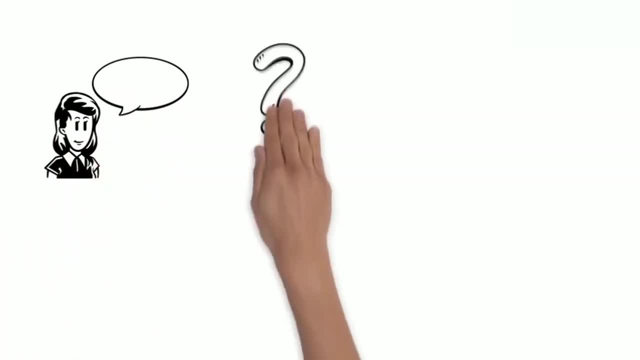 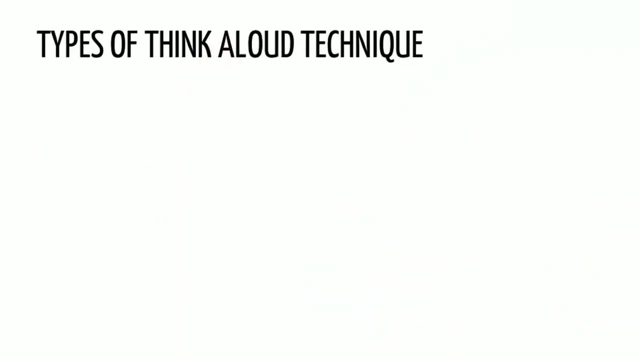 The participants are asked to not only tell what they are doing, but also why and what they think and feel while performing a specific task. There are commonly two types of think aloud technique: Traditional and retrospective. In traditional, participant speaks while doing the tasks. In retrospective, participants complete the task silently. 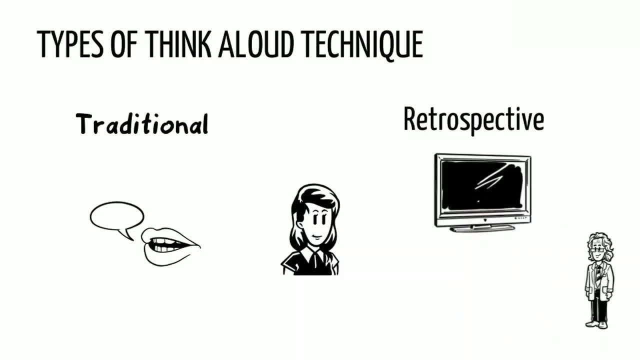 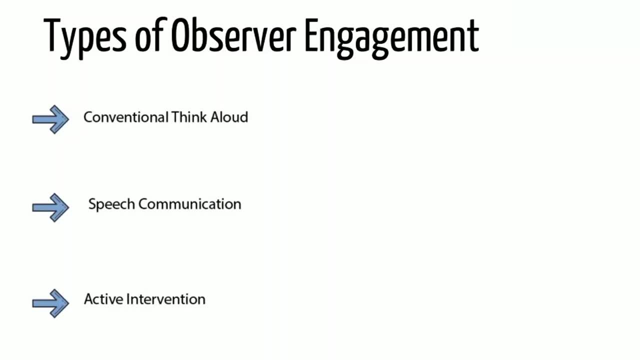 Then they reflect their thoughts while watching the recording with the researcher. There are three ways in which the researcher can act towards the participant: Conventional think aloud, speech, communication and active intervention. In conventional think aloud, the observer does not say anything. 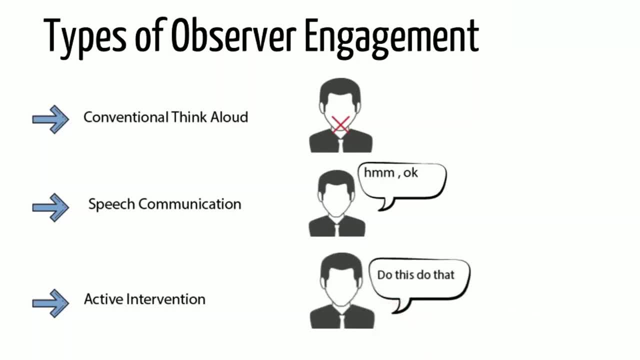 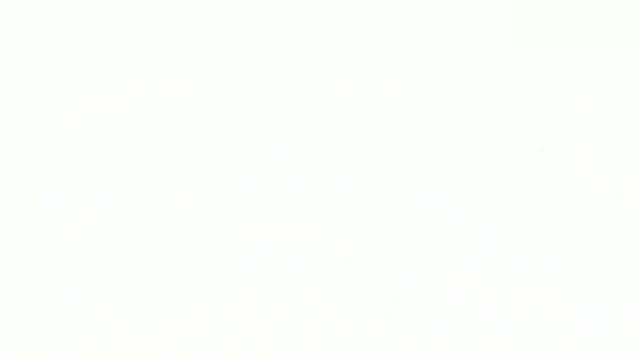 The observer responds with filler sounds, Whereas in active intervention, the observer intervenes if the participant gets stuck. This method is suitable within any step in the design process. However, it is particularly suitable during the early process, when the designer wants to evaluate the concept using a low fidelity prototype, such as a paper prototype wireframe. 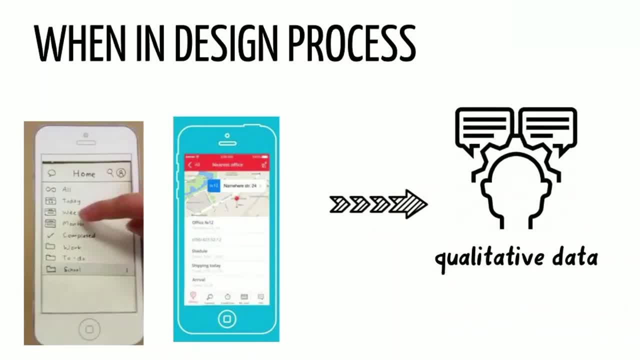 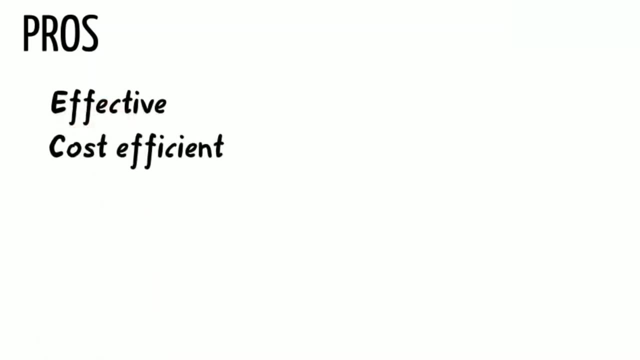 or early stages of a working prototype. The method gives qualitative data and shows if the user is able to understand what the element of an interaction is supposed to do. First of all, the think aloud method is highly effective and cost efficient. It is fast to learn and perform, and flexible as well. 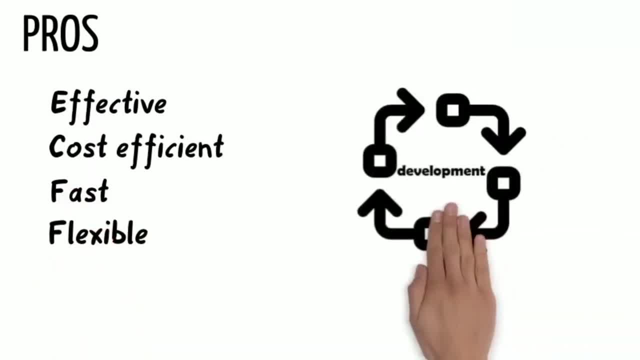 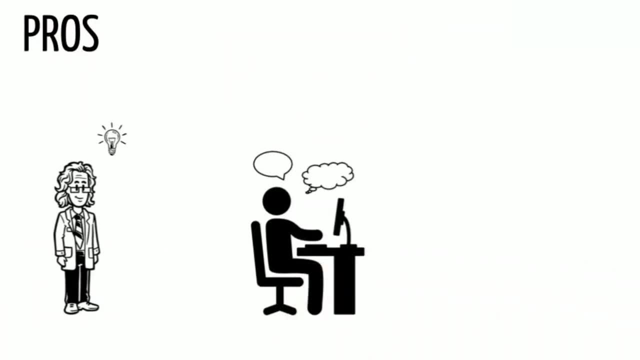 since the method is useful at any stage in the development process. The method gives an insight in the actual behavior of the participant while performing the task, rather than only the opinion. There are also some downsides to the think aloud method. Thinking out loud does not come naturally to most people.